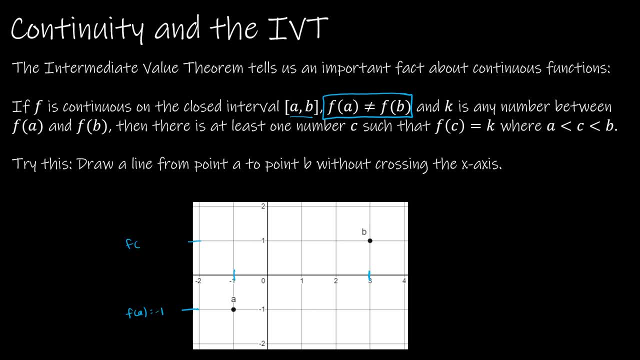 and k is some number between f of A and f of B. So f of A is negative 1, and f of B is positive 1.. Those are the y values. So we're saying if you have some value between negative 1 and positive 1, let's call it 0, but it could be any of the values in between. 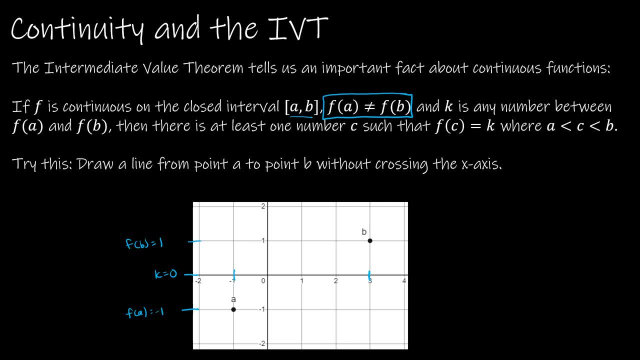 then there is at least one number, C, such that f of C is equal to k. So there's some number between A and B, between negative 1 and 3, called C. that f of C is equal in this case to 0.. So here's how. here's a good way to visualize what exactly. 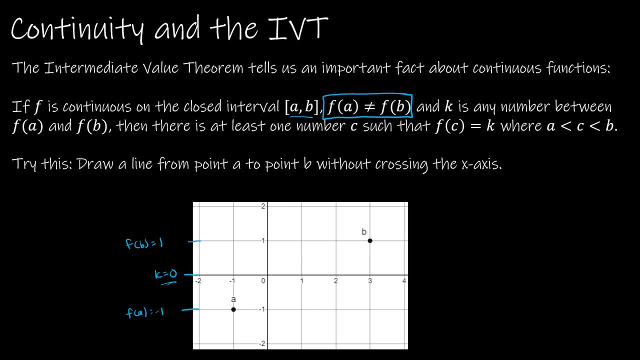 is happening. We're saying we've got two values, A and B, We've got their y values, f of A, f of B, k is some number between those, and f of A can't equal f of B. because here's why. 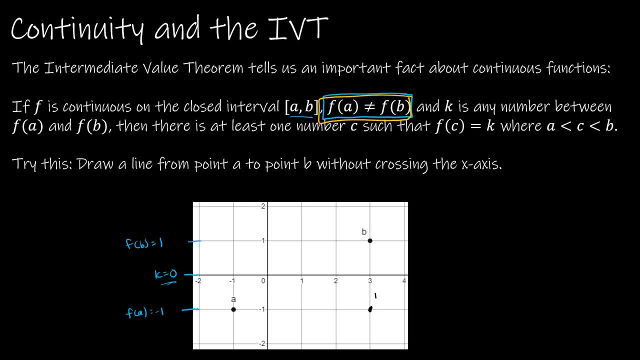 Let's say I put B right here, Then my little example won't work. It says: try to draw a line from point A to point B. If you draw a line from point A to point B, you can draw a line from point B to point B. 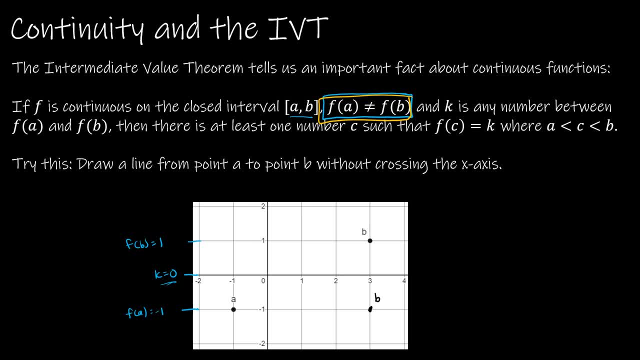 without crossing the x-axis. Well, if these two are the same, that's real easy to do. f of A can't equal f of B, because it doesn't guarantee anything. I could just have a constant function. However, if f of B is up here at 1, and f of A is down here at negative 1,, 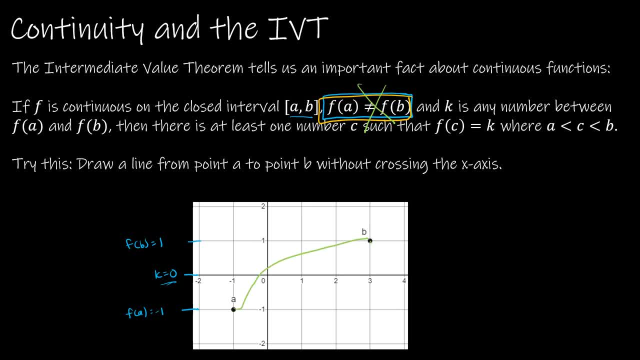 can I get from A to B ever without crossing the x-axis? Can I draw a continuous line of any kind without crossing the x-axis? No, I keep trying and I keep failing. I can't get from A to B without picking up my pen. 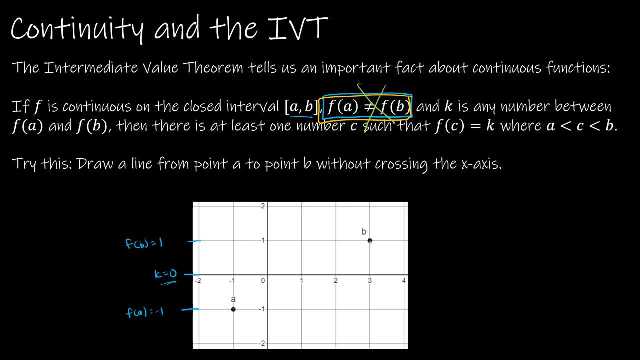 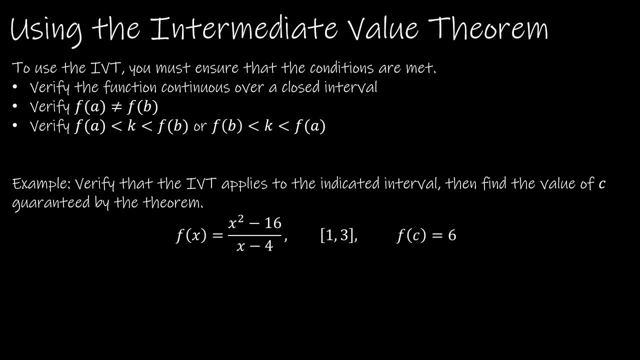 without crossing the x-axis. That's what the intermediate value theorem tells us. Before we talk about when the IVT can be incredibly useful, let's just do a practice to make sure we understand exactly how to use it. So, in order to be able to use the 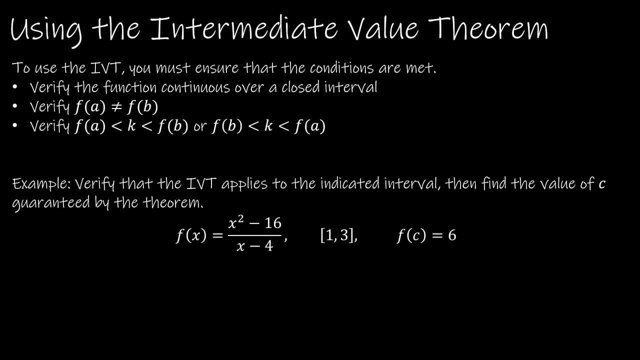 intermediate value theorem. you have to ensure that the following conditions are met, and I do expect you to actually show the following conditions. I'm going to show you the following conditions and I'm going to show you the following conditions. First, you have to verify that the function is continuous over a closed interval. 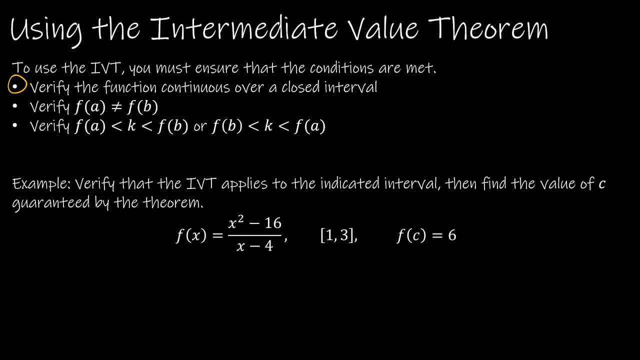 This is where that slide will come into play- that we looked at rational functions and radical functions and trig functions and knowing exactly when they are continuous or discontinuous. Next, we have to verify that f of A does not equal f of B. We already talked about why that's. 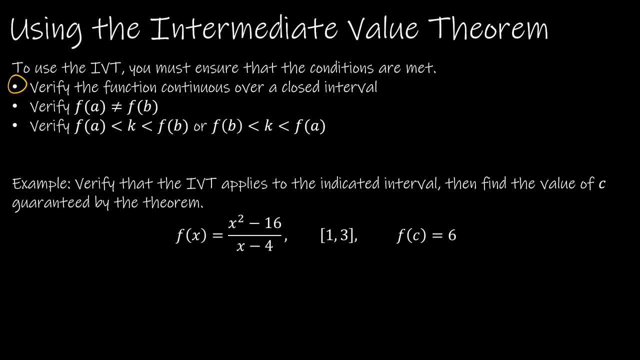 important, That's to ensure that we don't have some constant function. So verify that the two endpoints don't equal each other. And then we have to verify that the two endpoints don't equal each other. And then we're going to verify that f of A is less than k is less than f of B, or f of B is less. 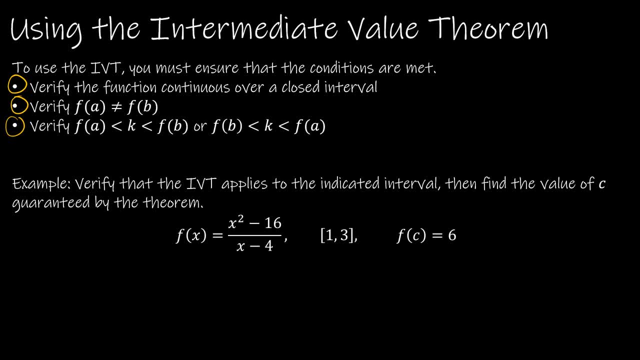 than k is less than f of A, which essentially says: make sure k, which is the y value, falls between f of A and f of B. So let's look at a practice together on exactly what kind of work that you would want to do to use the intermediate value theorem. So this says: verify that the intermediate 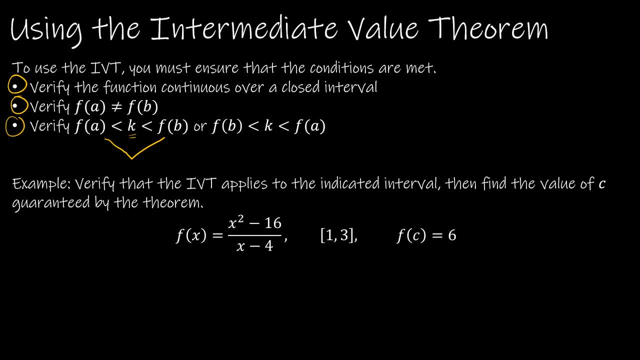 value theorem applies And then find the value of c guaranteed by the theorem. So to do that, essentially I'm going to be checking these two conditions. So I'm going to say one: verify the function is continuous. So f of x is not continuous. oops, is discontinuous at x equals four. because again we're looking at 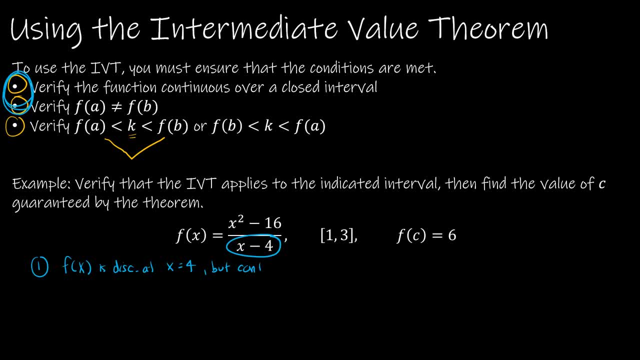 that denominator, But continuous on the interval 1, 3.. And that's the interval that's being given to us, So we're okay. Verify it's continuous on the closed interval. Verify that f of A does not equal f of B. 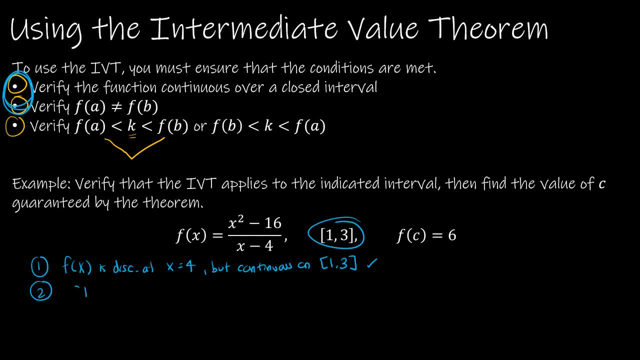 So one, let's do f of 1, because 1 is the left-hand endpoint. So that's 1 squared, which is 1 minus 16 over 1 minus 4.. That gives me negative 15 over negative 3, which is 5.. And f of 3,, which is the right endpoint, would be 9 minus 16 over 3 minus 4, which is negative, 7 over negative 1, which is 7.. 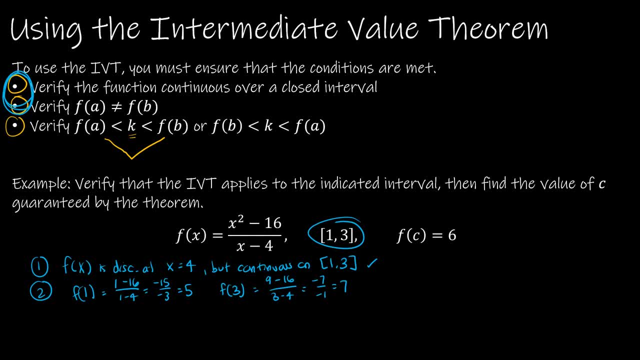 So 5 and 7 are the two endpoints. So f of A does not equal f of B. And the third condition is that the point that we're looking for, f of C, does not equal f of B. So we'll say f of 1 is less than f of c, which is 6, is less than f of 3.. 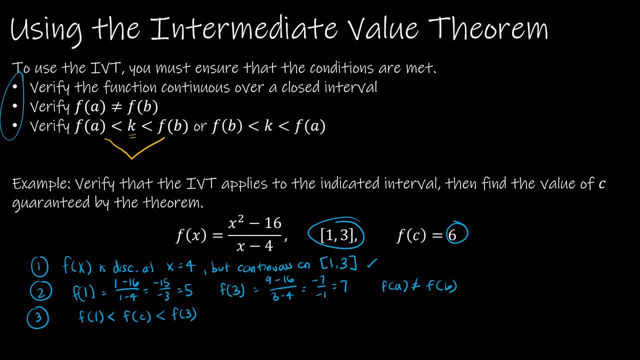 So really I've checked all three of those now: 1,, 2,, 3.. Then I have to actually find the value of c guaranteed by the theorem- Ooh, that yellow is a little bit obnoxious. Find the value of c guaranteed by the theorem. 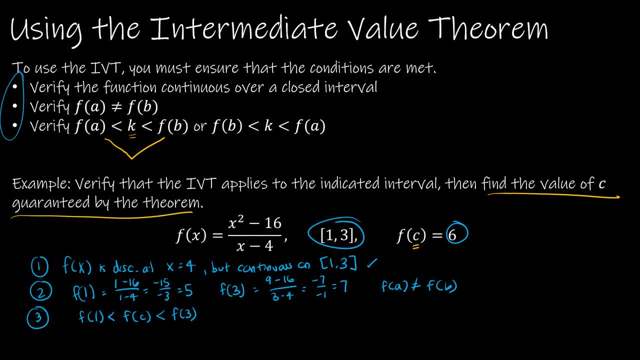 So what that means is solve for when f of c is equal to 6.. So x squared minus 16 over x minus 4 has to be equal to 6.. So now it's just algebra: x squared minus 16, I'm going to multiply each side by x minus 4, so that's 6x minus 4.. 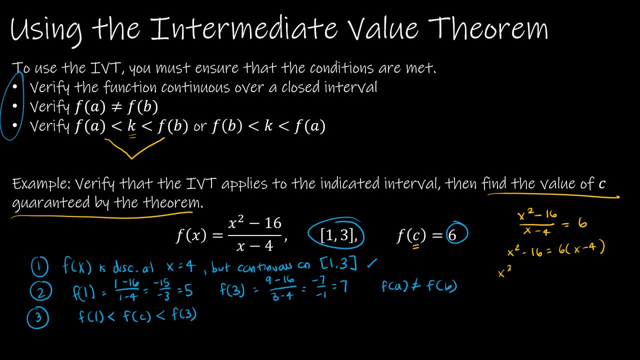 This is obviously a quadratic, so I'm just going to plug everything over to the left side, So that's x squared minus 6x. This side would be minus 24.. I would add it over, so that's plus 8.. 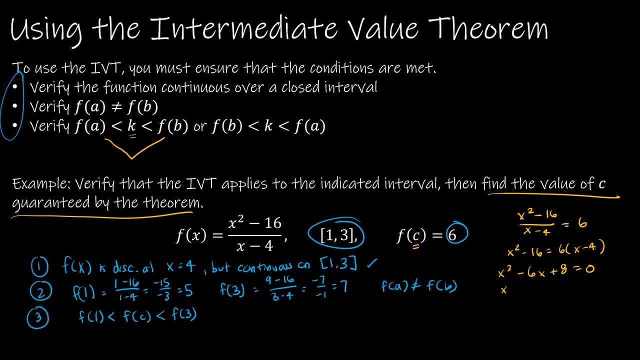 And then this would be x minus 4, x minus 2.. So x is 4 and x is 2.. However, remember, I'm in the interval 1 to 3, so I really only care about the x is 2.. 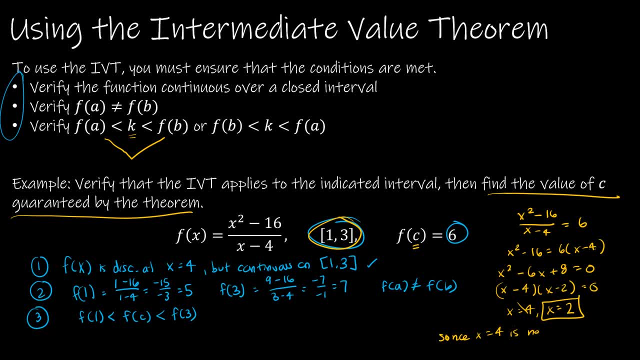 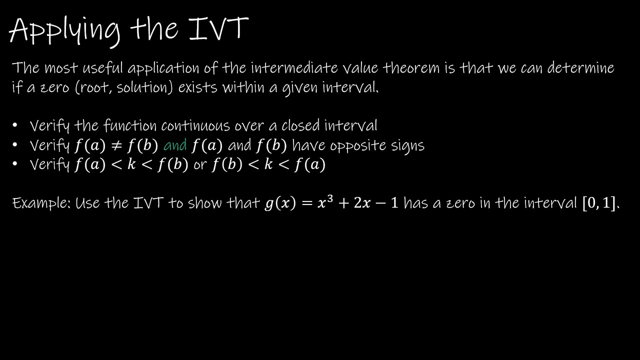 Since x equals 4 is not in the interval, then c is equal to 2, and f of c is equal to 6.. The intermediate value theorem: all by itself not super helpful, except for when we can apply it to determine if there is a zero or a root or a solution. 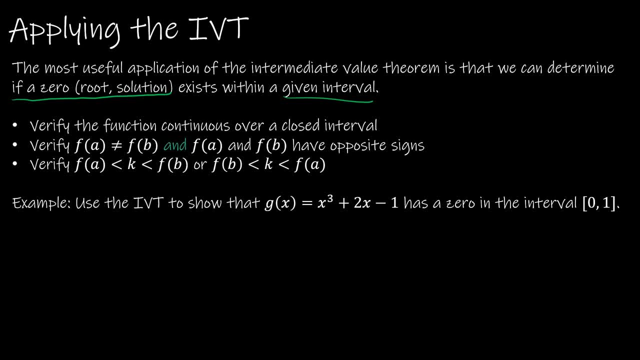 within a given interval. That's when we use the intermediate value theorem the most. So notice, I'm going to do the expression. the exact same thing I did on the last question. The only difference is I have to ensure that f of a and f of b have opposite signs. 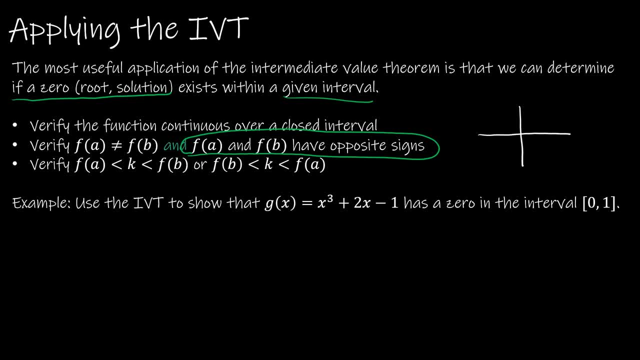 And again, the reason for that is if I know that f of a and f of b have opposite signs, then in order to connect those two points, I have to at some point cross the x-axis, which is where the zero, or root, or solution will occur. 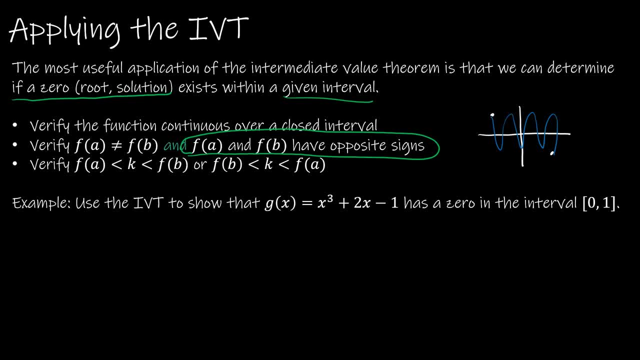 So it might occur more than once, but I know that in order to get from point a to point b, I have to cross over the x-axis. So you have to also include that f of a and f of b have opposite signs. So let's take a look at how this would work. 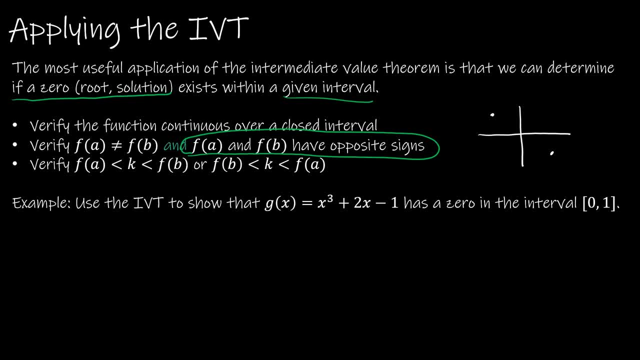 We're asked to use the intermediate value theorem to show that g of x is equal to x cubed plus 2x minus 1 has a zero in the interval 0 to 1.. So 1.. g of x is continuous. It's actually continuous everywhere, but I'm going to say over 0, 1.. 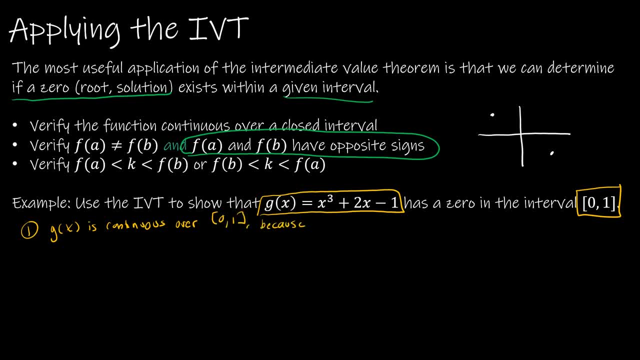 Because that's the interval, Because g of x is a polynomial. So again, that's where that review comes into play, where we know polynomials are continuous everywhere. 2. Verify that f of a does not equal f of b. So again we're looking at 0 and 1 for a and b. 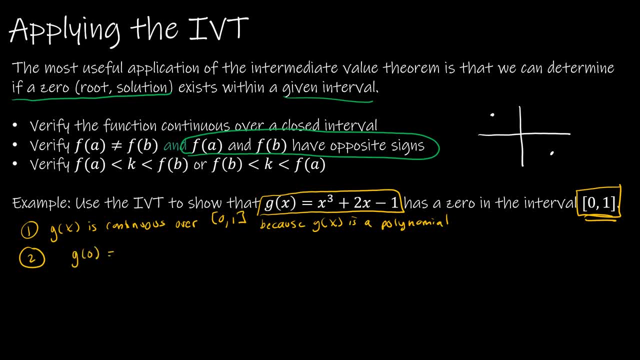 So g of 0 is 0 plus 0, minus 1, or negative 1.. And g of 1 is equal to 1. Plus 2,, which is 3., Minus 1,, which is 2. So g of 0 does not equal g of 1.. 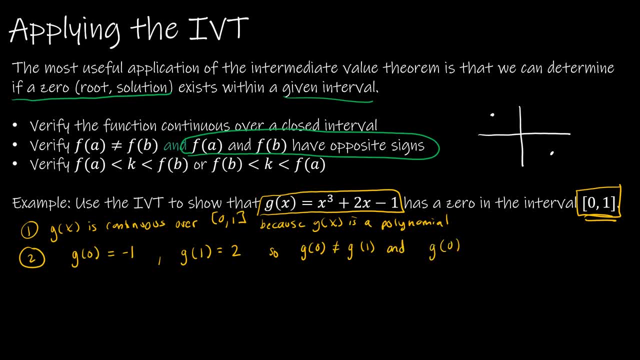 And g of 0 is less than 0, so it's negative And g of 1 is greater than 0. So I verify that they have opposite signs. The last one says: verify: f of a is less than k. is less than f of b. 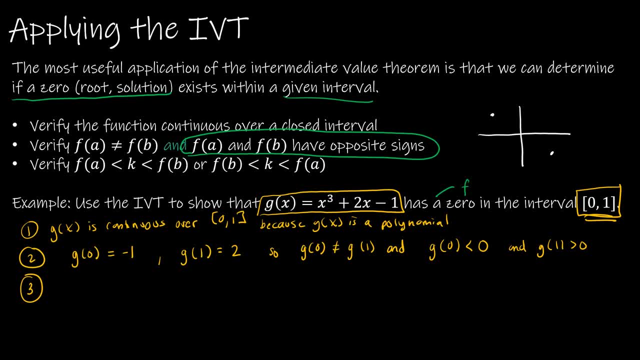 Well, this one's pretty straightforward. We're saying that f of c has to be equal to 0. So essentially, we're saying that g of 0 is less than f of c is less than g of 1.. And it could go in either direction, but we have to basically say that that value is between the two other values. 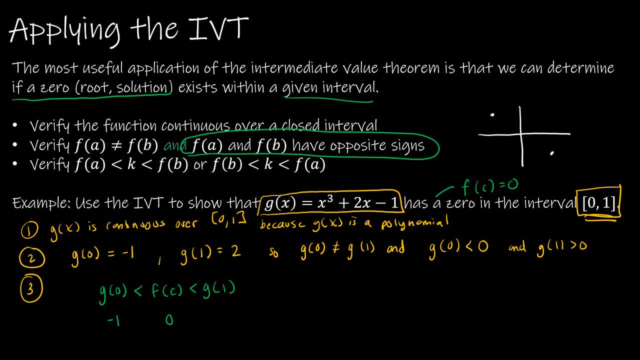 So g of 0, remember, was negative 1.. f of c is the 0. And g of 1 is 2.. So obviously this makes sense. g of 0 is less than f of c is less than g of 1.. 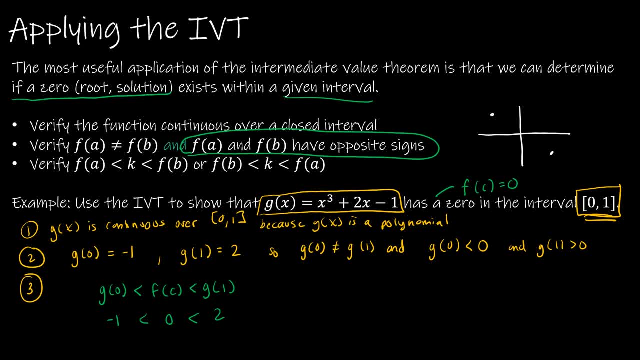 Now does it ask me to find the value of c? No, It just says: use it to show that there's a 0 in the interval. So therefore, there is a 0, or root or solution, in the interval 0 to 1.. 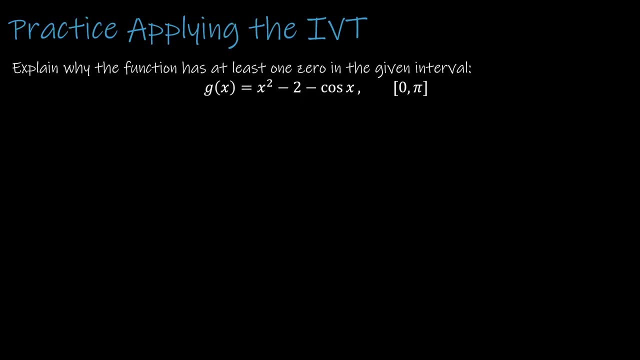 Here's a question for you to try on your own. So press pause, Try this question When you're ready. press play to see how you did So again. we're trying to just explain why the function has at least one 0 in the interval from 0 to pi. 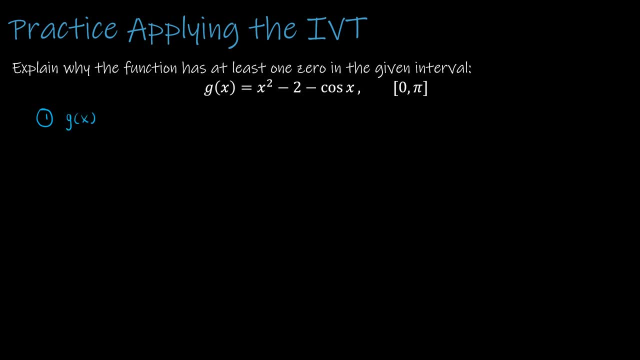 So first thing I have to do is say that g of x is continuous over the closed interval from 0 to pi. And again, why is that? Because each part, Each part, Each part of g of x is continuous everywhere. So we've got x squared, continuous everywhere. 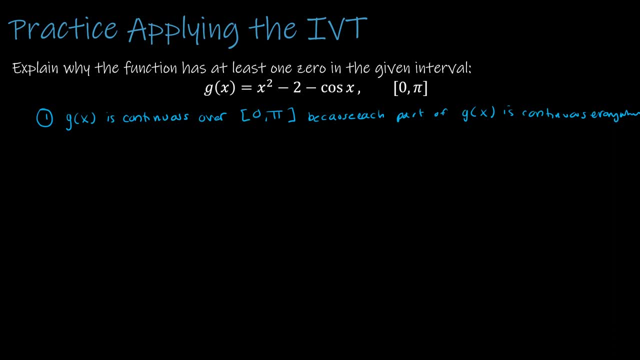 2,, I'm sorry, minus 2, continuous everywhere. Cosine of x: continuous everywhere. So that is how I would explain it. Part 2.. Let's find g of 0.. g of 0 would be 0 squared minus 2, minus cosine of 0, which is 1.. 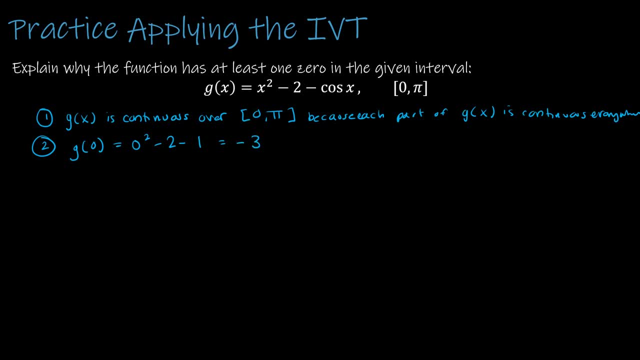 So that's going to give me 0 minus 2 minus 1 or negative 3.. g of pi is going to give me pi squared minus 2 minus negative 1, which is actually plus 1. And that's going to give me basically pi squared minus 1.. 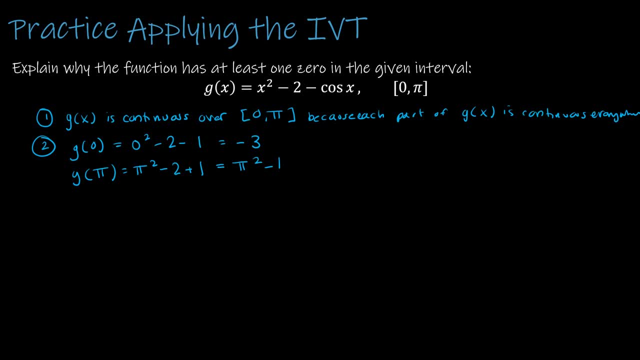 Now I don't need to know exactly what that is. I just need to know if it's positive or negative. So you can certainly use your calculator to figure out. It's about 8.8.. 696.. But essentially we need to make sure we know that it is positive.